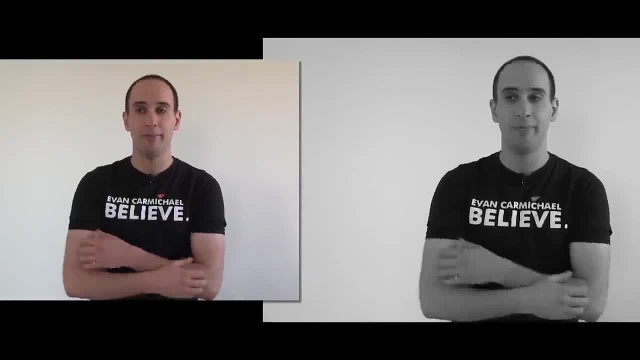 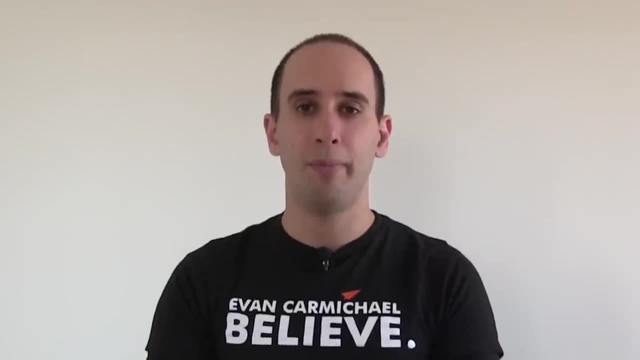 then they have a case for wanting to have a bigger piece of the pie. Regardless of the decision of how much percentage you're going to give up, you have to make them commit to the business. This is so important. I get that it's exciting at the beginning. okay, Partnerships are always exciting. 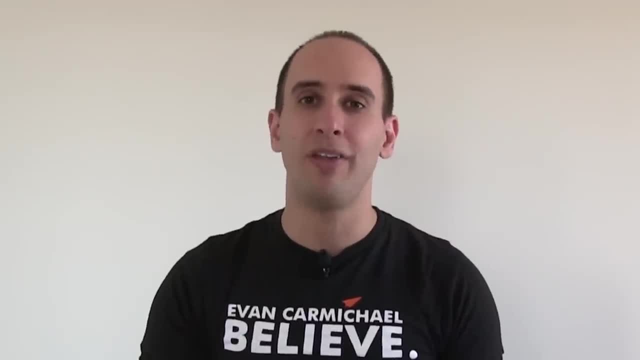 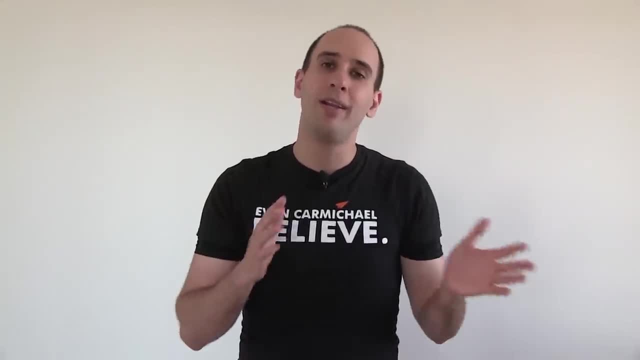 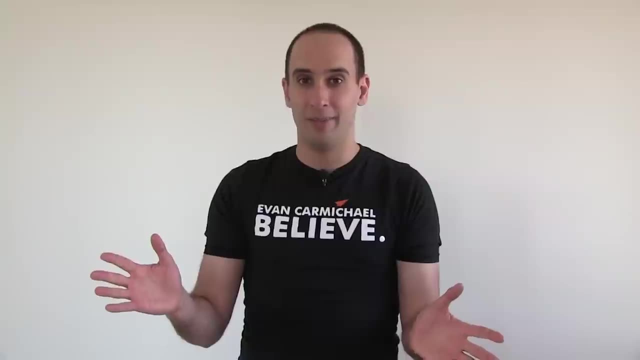 alone And it's just. there's so much pain of going alone and so much excitement of bringing somebody new on that. all you see, is the good side. Not a lot of partnerships will work out all the way to the end And you want to make sure that you're really getting the right person on. 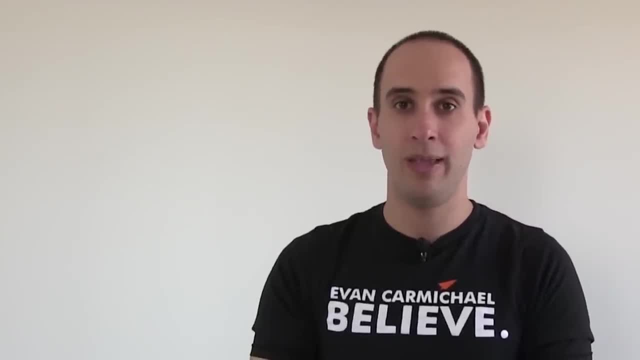 board. It really is like choosing a spouse. Okay, you have to know them, like them, trust them, love being around them and think that it's going to work out for many, many, many years. And what do you do before you get married? You date. 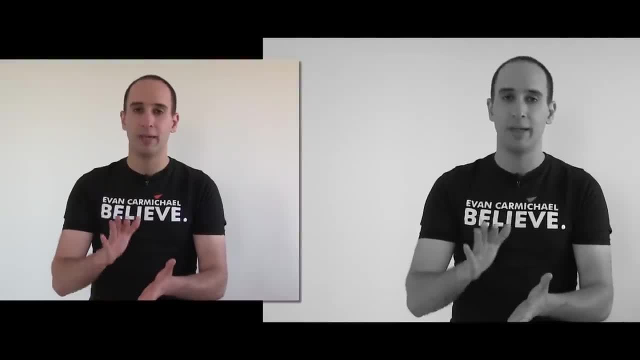 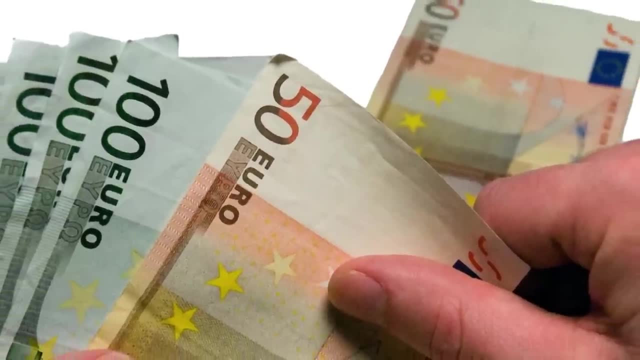 And that's what you need to do with your business as well. You need the person to commit to the company before you just give them equity, And that can come in two forms. One: they buy in, They have to pay. They have to pay for equity in your company. Your business is worth something. 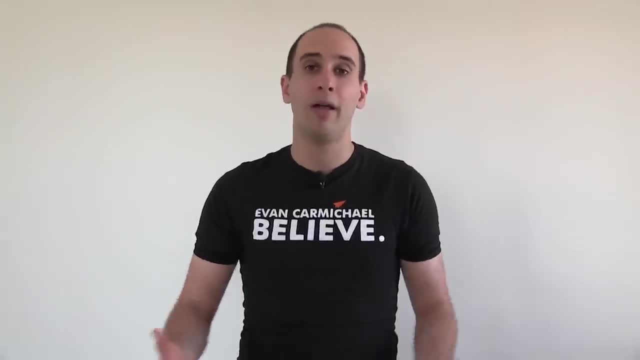 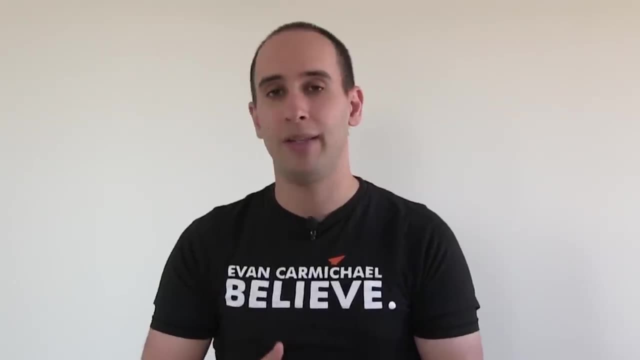 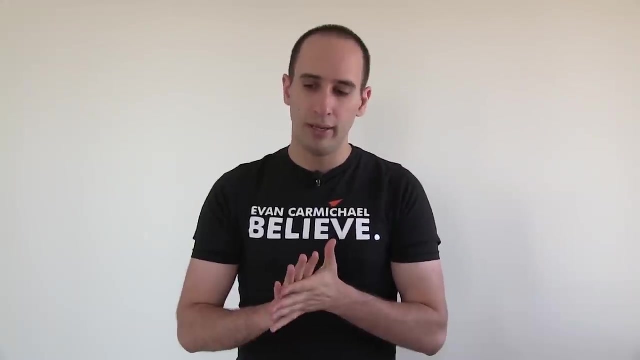 and you're not just going to give it away. They have to buy a certain amount at a certain price. The other way is to earn in, And so, instead of just giving them X percent of the company, they earn it when they hit milestones. So I remember I had a software company when we 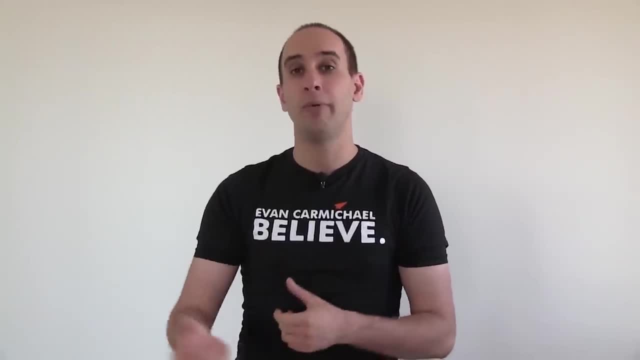 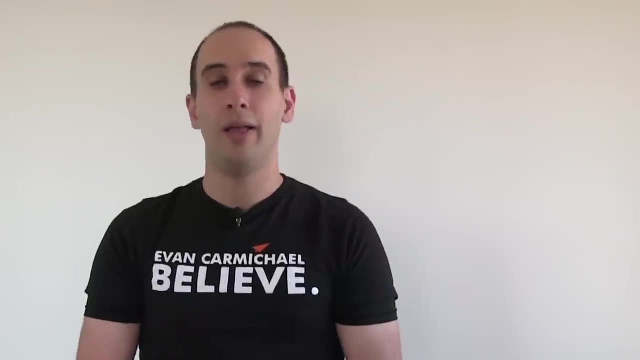 were bringing on a new salesperson. It was started by myself and my business partner. We're bringing on a third partner who's going to be our salesperson And he was joining relatively early on, but I didn't know him too too well And I didn't want to just give him a piece of my company. 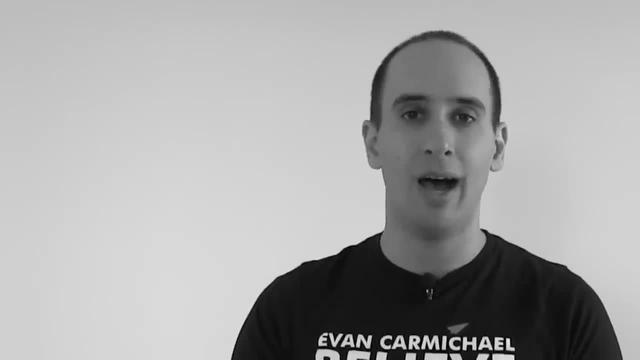 because the last thing you want to have happen in your business is have a company that's going to have a guy who owns a piece of your company, who's just a dead weight, who isn't doing anything for the company and is somebody who you don't want to be around. And that can happen very often with a 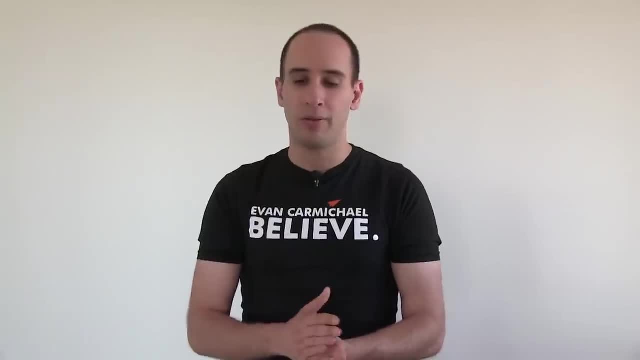 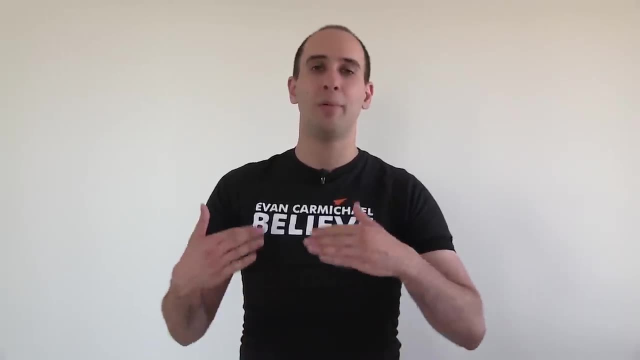 lot of companies. So we made him earn in and we said, okay, we'll give you up, to whatever it was, 20% of the business. You earn your first 5% if you can close X number of deals within this amount. 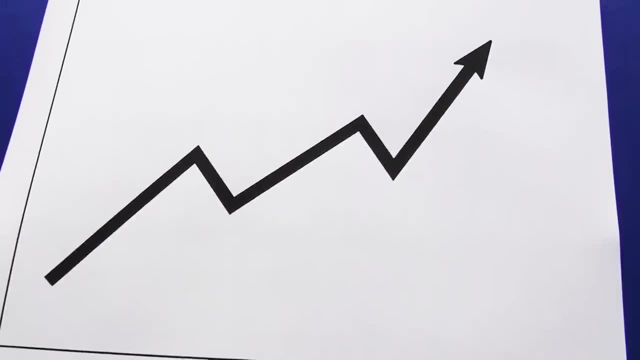 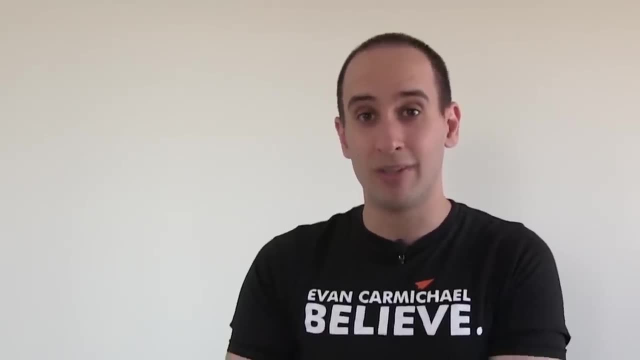 of time And we set milestones So you get your first 5% when this happens, your next 5% when this happens, And so it shows that they're- they have to be committed to the business and actually get results for you before you're going. 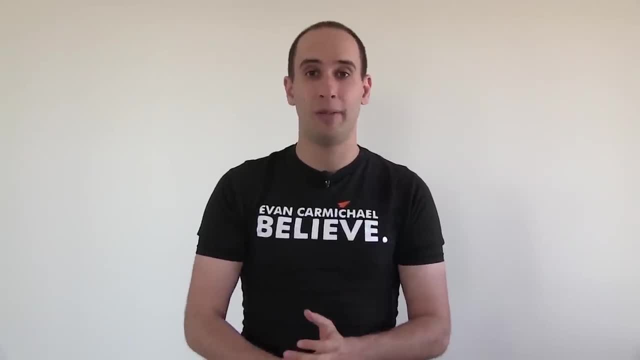 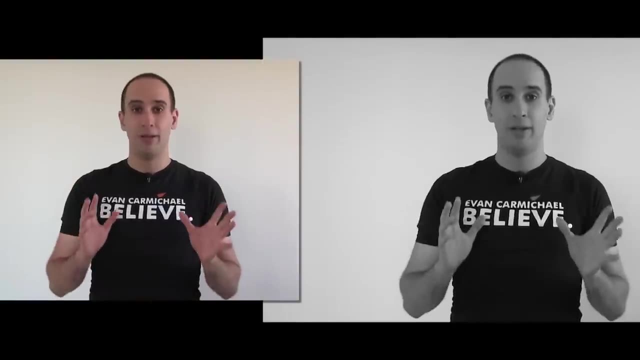 to give them equity. So I would encourage you to have some kind of benchmark to put in. if they're not going to be buying in and giving you money for your shares, The last thing I'd encourage you to do is for anybody who's bringing on a partner is have a shareholder's agreement. It's so important. 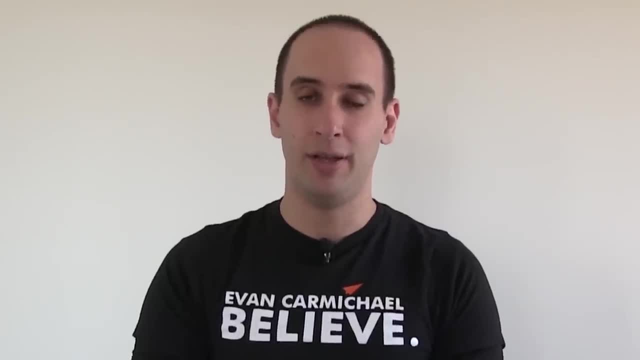 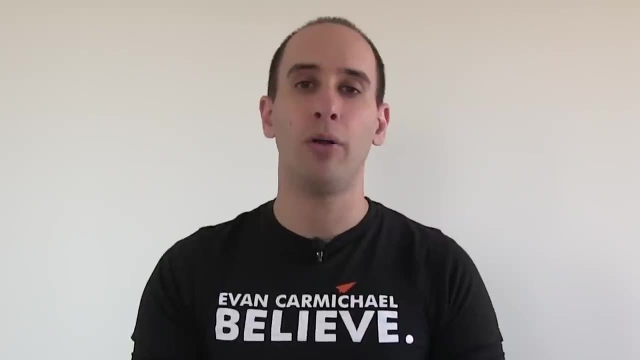 and make sure that you include a shotgun clause. A shotgun clause, basically, is something that you write into your shareholder's agreement that allows one person to have a shareholder's agreement. It allows one partner to buy out another partner. if it's not working out, You know, for whatever. 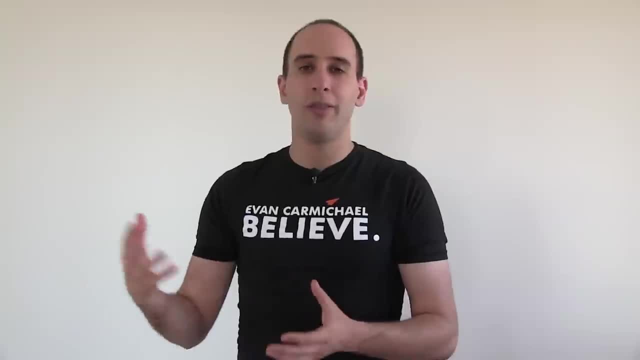 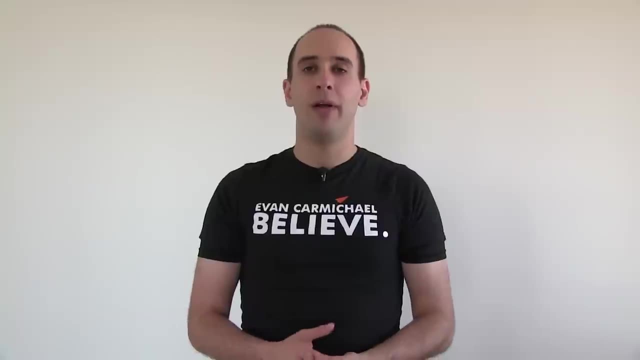 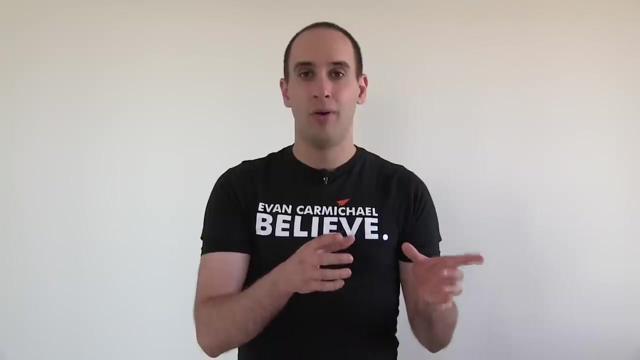 reason. it's just not working out. You're fighting, you're doing all the work and this person's not doing anything. and they own 50% of your business. How do you get them out? And a shotgun clause says: I will buy your shares at this price or you have to buy all of my shares. 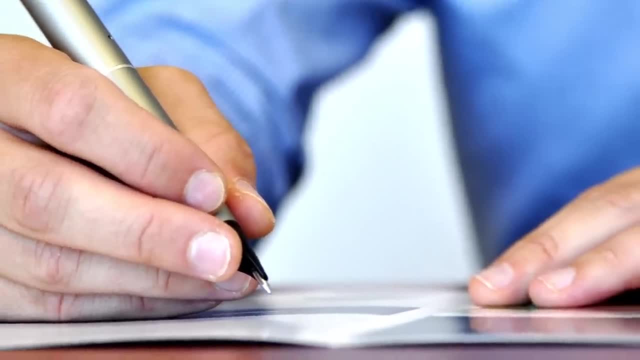 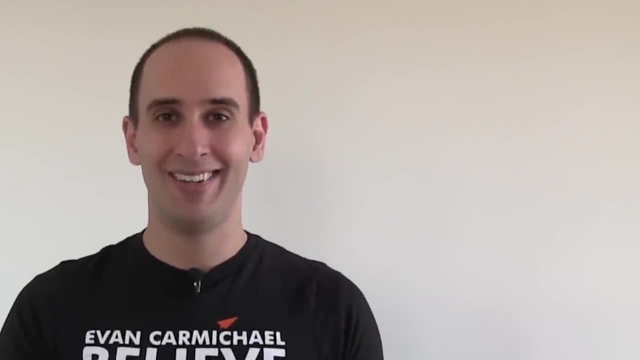 at the same price. So you get to pick the price and the other person gets to pick the price. So you have to either accept the deal or buy you out. So one way or the other somebody is getting bought out of the business. So you have to be smart with what price you set. 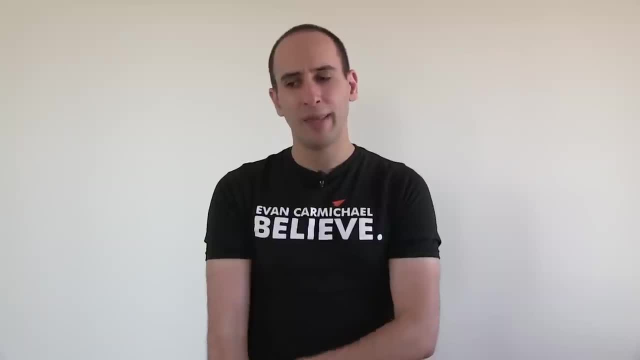 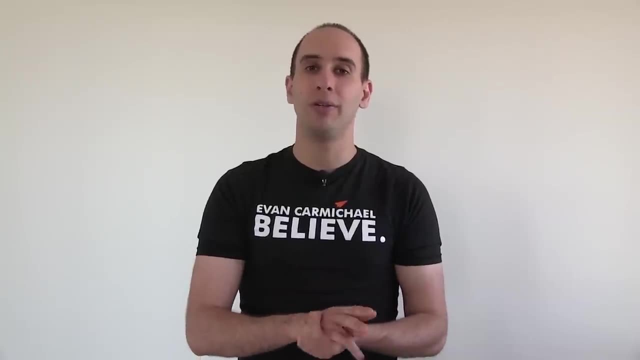 but it's an important part to have in your shareholder's agreement before you bring on a partner. The other thing you might want to look at is a piggyback clause, And that's basically where, if one person is a minority shareholder, if you decide to sell, that person can come with you. 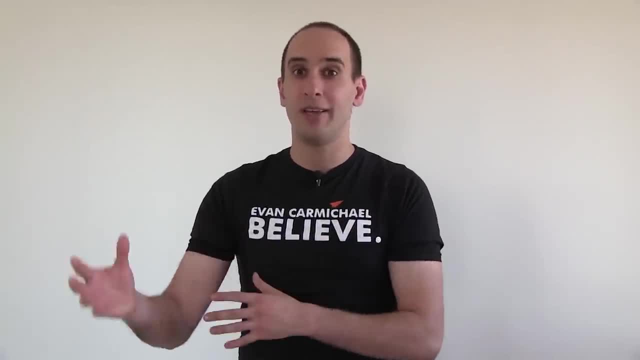 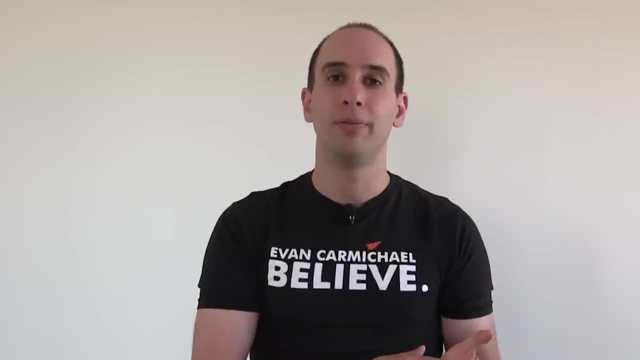 So you know if you're the majority shareholder, so somebody who's a minority shareholder you sell your business, that person has to go with it, So you don't have one person holding up a deal. So if you have a deal to sell your company, that minority shareholder can cause a lot of. 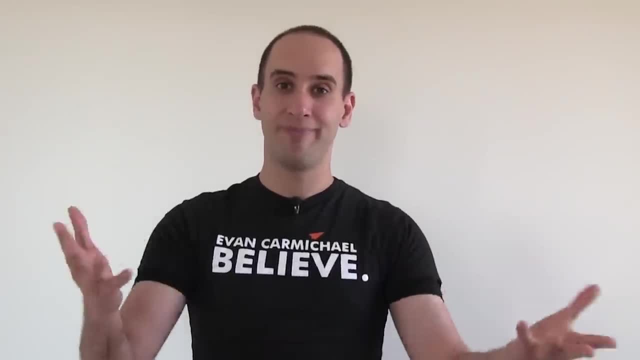 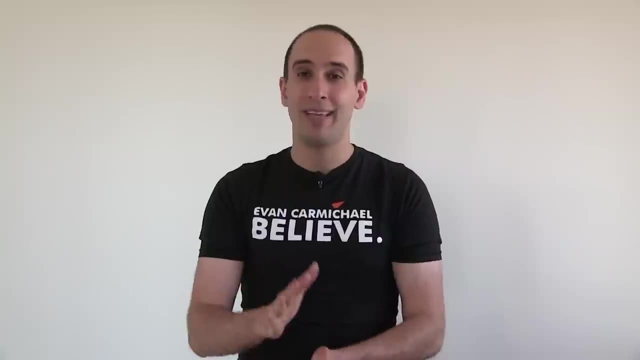 problems for you and prevent the sale of the business, which you know you don't want to have happen. So that person is dragged along with the sale of the company. Anyway, a few things to think about. get a lawyer involved, but you definitely don't have to give up 50% of your.